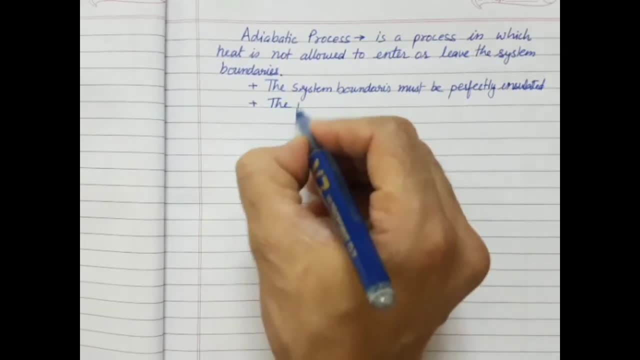 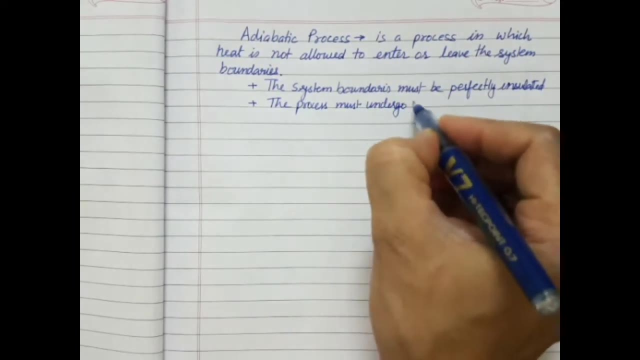 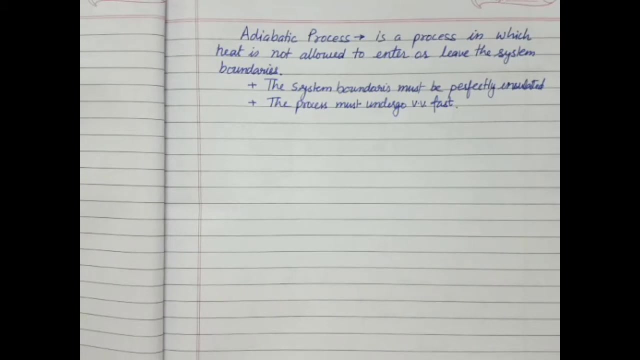 number two: the process must undergo very, very fast. So these are the two main conditions to achieve the adiabatic process. why we put song conditions? because in adiabatic process the heat energy is not allowed to enter or leave the system, as per definition. so delta q is equal to zero. 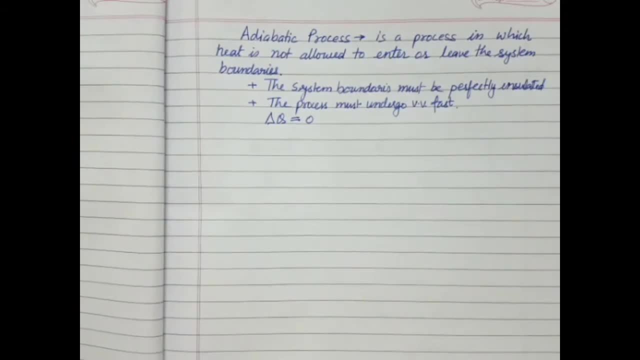 initial def was given. delta q means 0.. future is 0.. is any process if we compress the gas within a confined space now? during compression there must be a change in internal energy of the system, So heat energy will be evolved from. 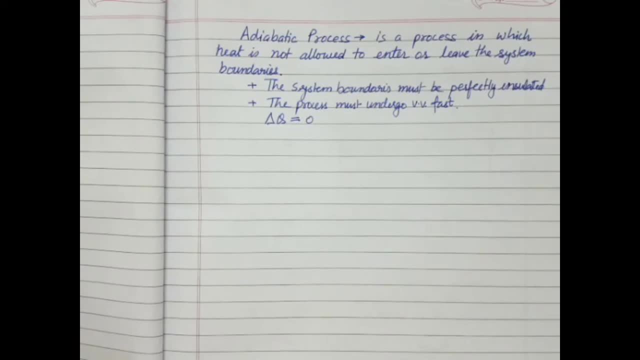 the gas. Now, if the system boundaries are not, you can say they are not perfectly insulated. the heat evolved will conduct it out of the cylinders, It will conduct out of the system boundaries and what will happen? that and the temperature will move and this load in. 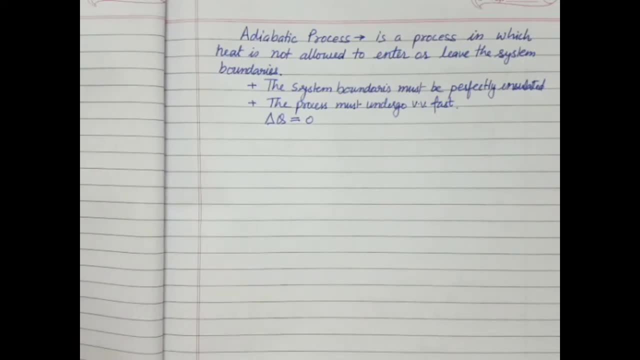 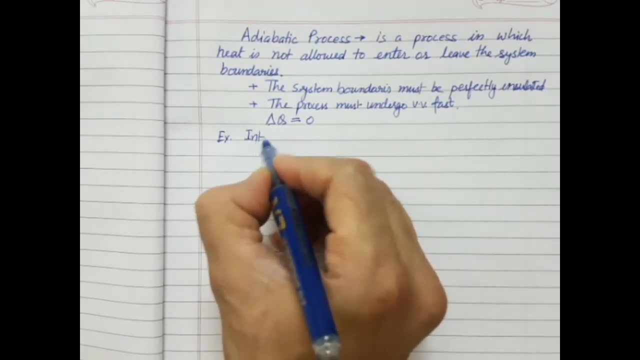 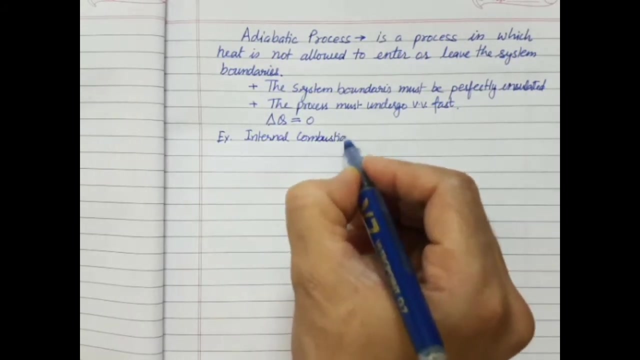 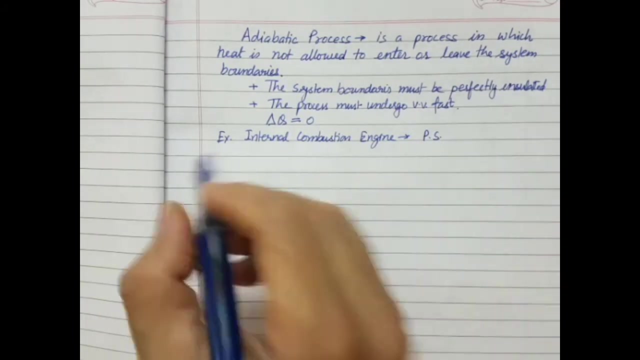 the system, So it will defy the conditions of adiabatic process. So to achieve this process, the system boundary should be very perfectly insulated. Now, the very good example of this process is internal combustion engines. Now what will happen during power stroke? We burn some fuel in within a you can say: 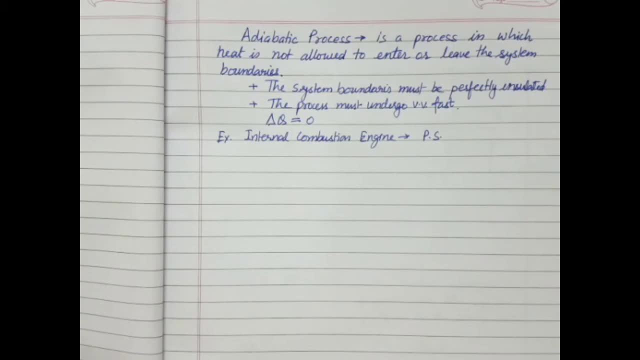 compressed. when the fuel air flow mixture is compressed, there is a spark and the fuel is burnt. At that instant, lot of heat is produced inside the piston and cylinder arrangement. Now this heat we try to achieve. we try to convert all of this heat into effective 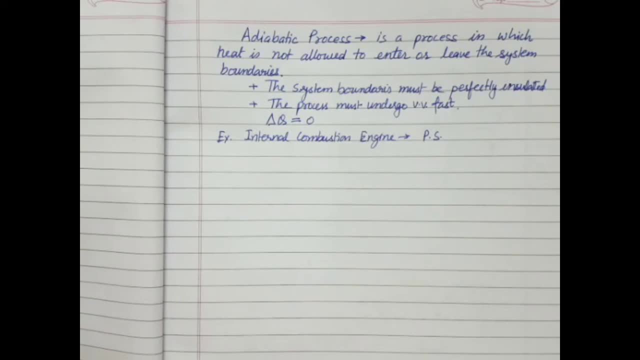 work. So to achieve this, we need to make this process very, very fast And, moreover, we want that no heat should be, you can say, wasted or no heat should be leak out of the system. So for that we also need very insulated boundaries, But in case of ice engine, this 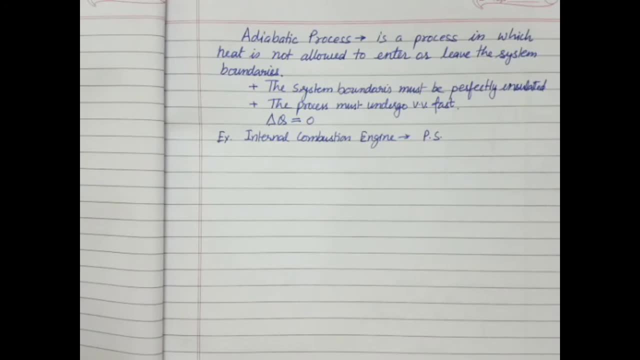 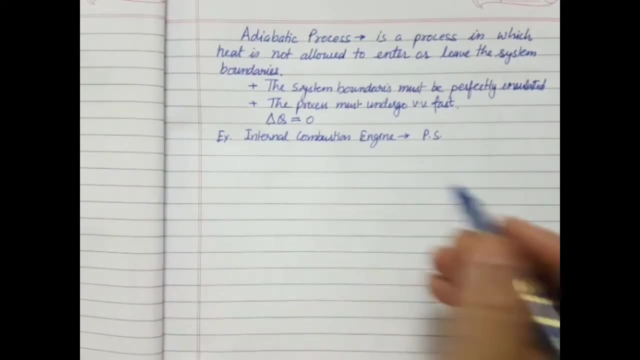 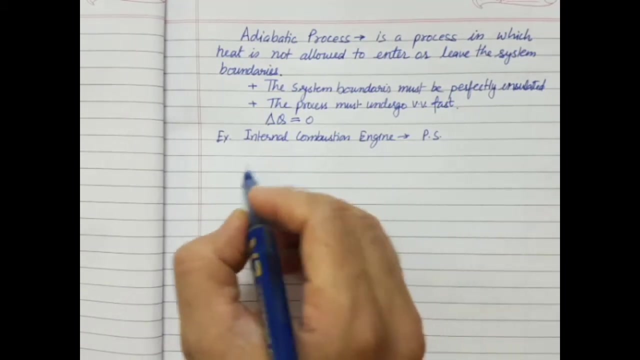 may not happen, but the process is very, the process made is very fast, So that we can achieve the adiabatic process. Now let us do, and this calculations for it, it's various equations. Now we can draw adiabatic process. 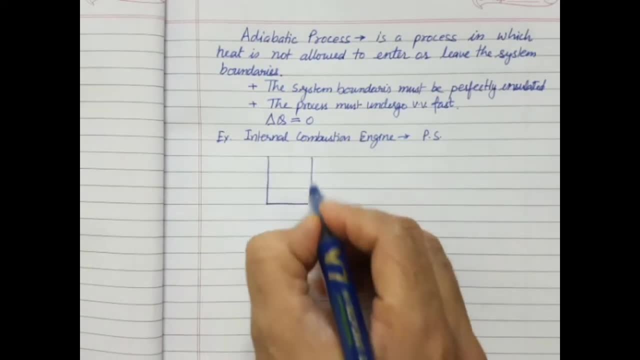 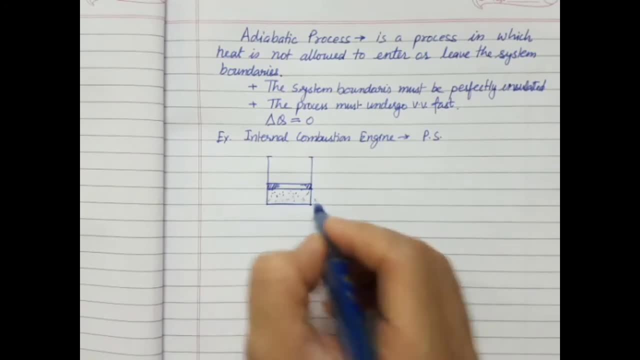 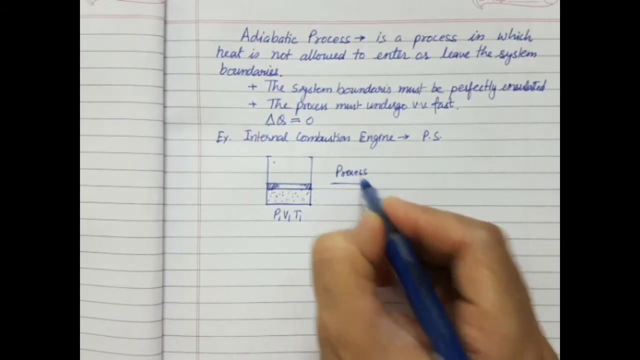 There is a gas inside the piston and cylinder arrangement And let us say here the coordinates at one. this is p1,, v1, and t1.. Now there may be some process occurring in the system like, let us say, compression, this power stroke. 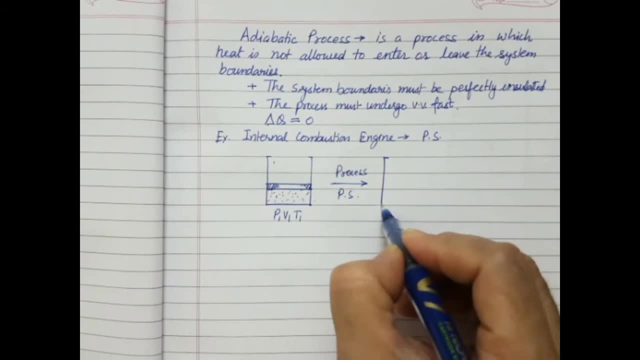 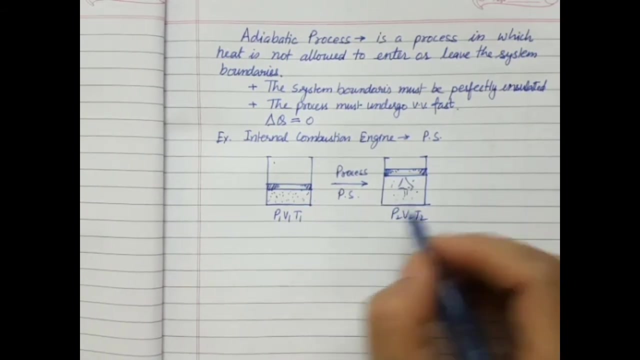 So during power stroke the piston will move backwards So it may move up to this point. So due to, you can say, expansion of gas. So coordinates become P2, V2 and T2.. Volume pressure, temperature, everything changed. So during this process no heat energy is. 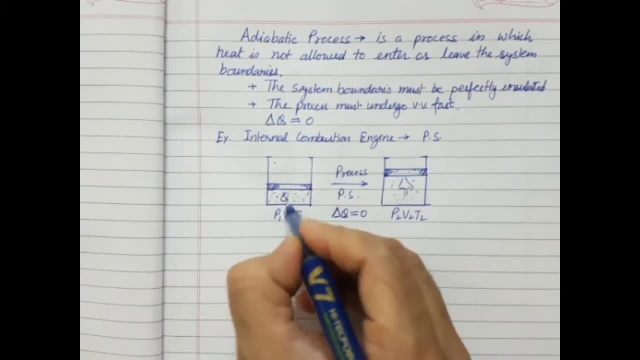 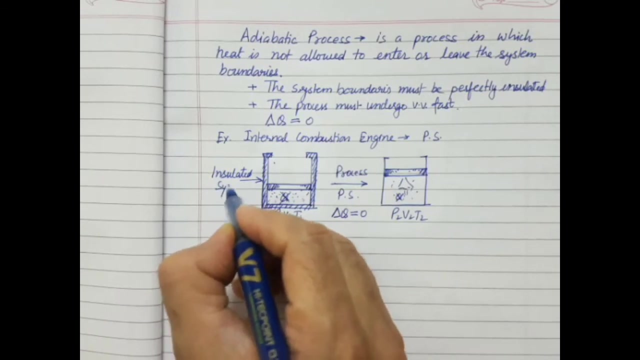 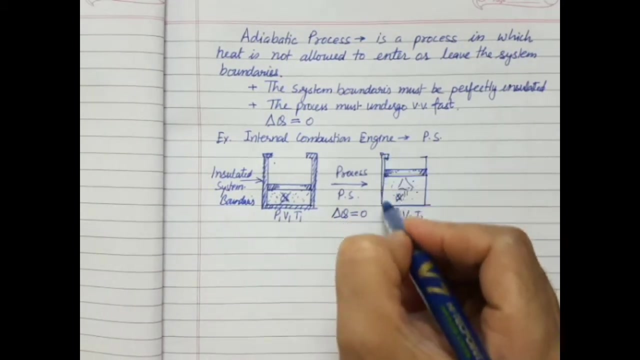 allowed to leave the system. So delta Q is equal to 0.. Q cannot leave the system. Here also Q cannot leave the system. So the system boundaries are insulated, perfectly insulated boundaries. So you must draw system boundaries. Here again we can draw similarly perfectly insulated system boundaries. 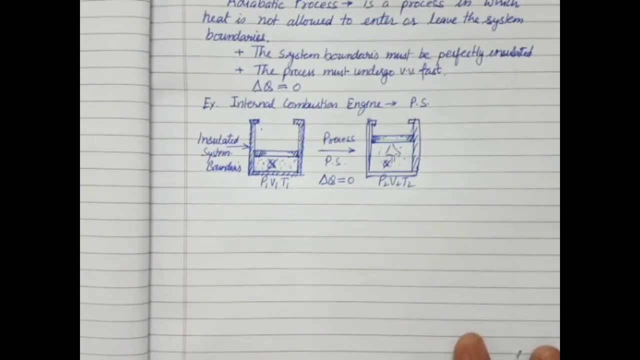 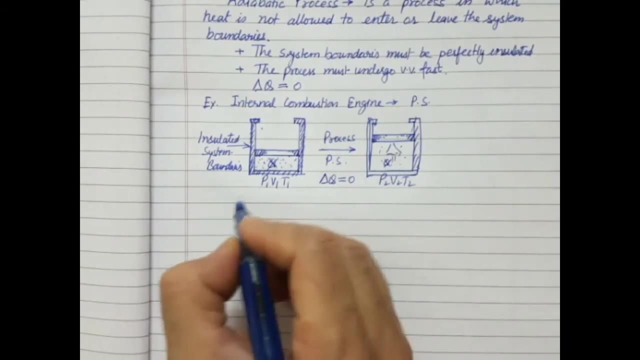 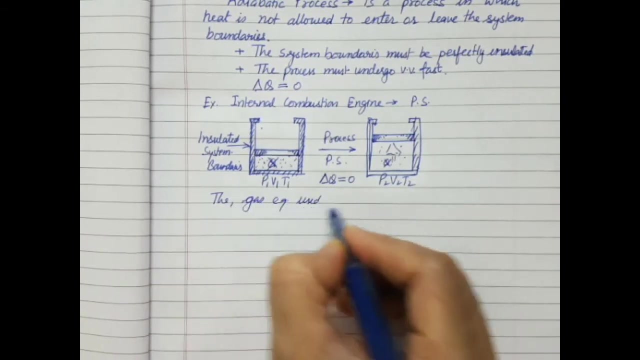 So this is your system. So now, let us Now, in this case, the gas equation used. the equation, the gas equation equation used is P V raised to power, gamma is equal to constant. Now, how this equation comes, you can see. 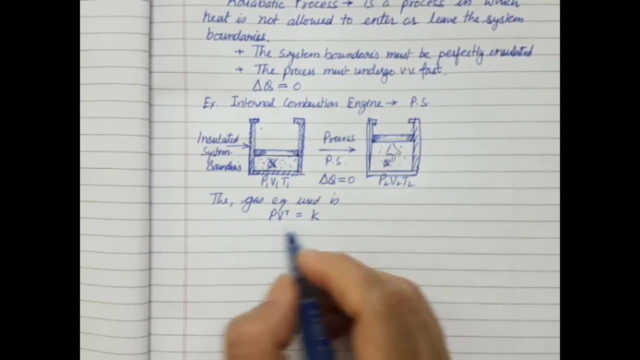 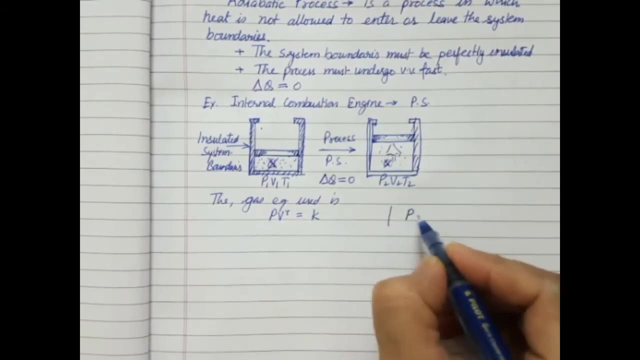 in the book. We will not go into that detail, But let us start from this equation. Now we also know that P V raised to power gamma is equal to constant. So P V raised to power gamma is equal to constant. Now what we have to do is we have to write this equation. 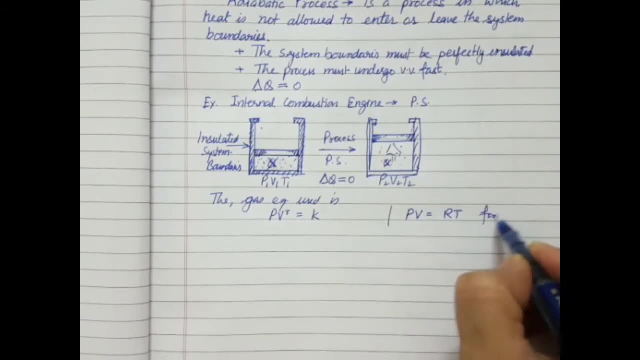 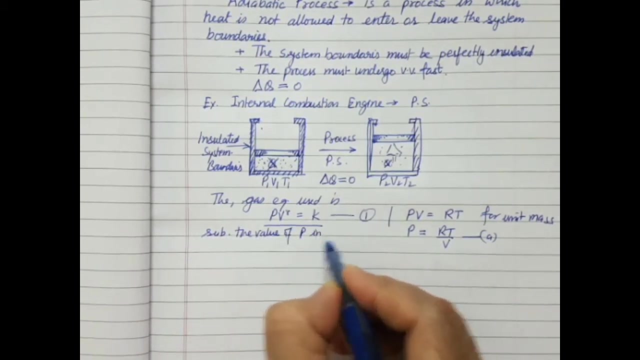 like that. this is equation 1. now substituting the value, value of pressure, P in equation 1. now what we get? we get RT over V. this is P multiplied by V. gamma is equal to. 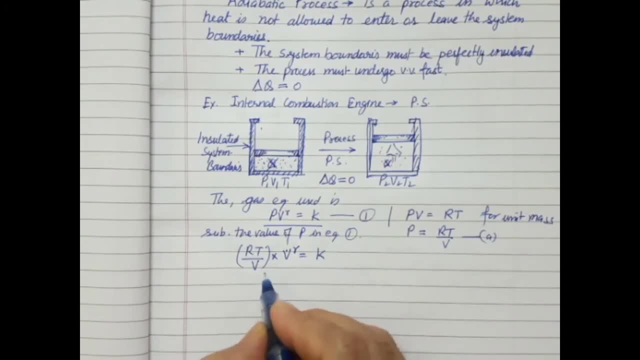 constant. now here again, R into T, into V gamma minus 1, V gamma minus 1. from this V minus 1 is equal to constant. now here R is constant and this is constant. so we can rewrite this equation like: T times V gamma minus 1 is equal to constant. so 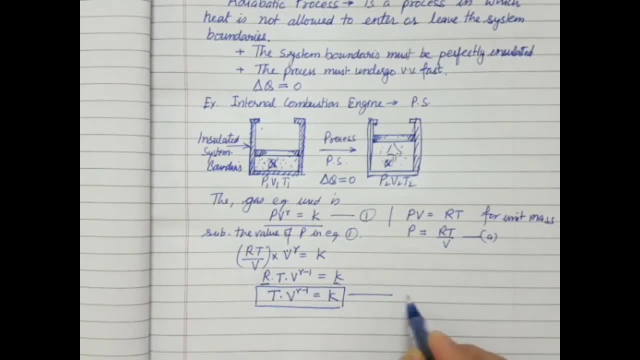 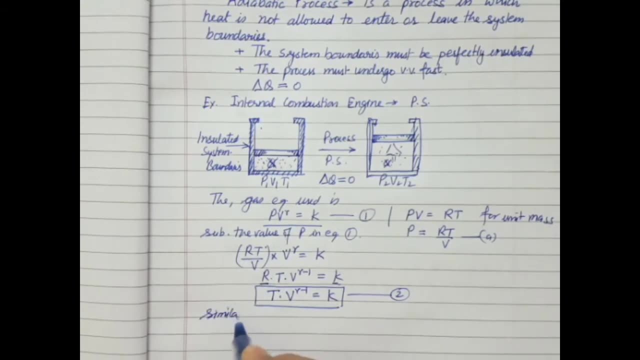 this is another equation we will use while doing analysis for the work done, similarly in terms of temperature and volume. similarly, we can also find the equation for in terms of: from here, like volume is equal to RT by P, this we can get another equation, equation in volume and temperature, in, in, in, in, in. 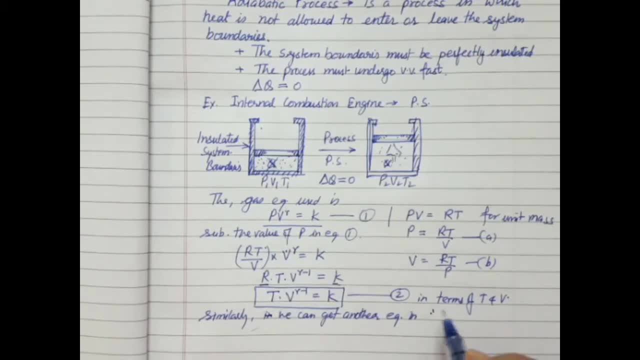 pressure and volume. so again, PV gamma is equal to constant. Now this is just. the question is in other equation should be any else we differently apply. so with this we are going to put that evaluation, a vector from equation. the value of very, so we get V is equal to RT by P from equation. b, so we get a grade of value 4. 그다음에 this asset stands for just 3 in 3, or if the results form horizontal or decimal position. so we get P into RT by. P is equal to the vector. So this is liquid value, which is a Van degli equation. b square by zero, by 3, 1 minus R, to gamma V. 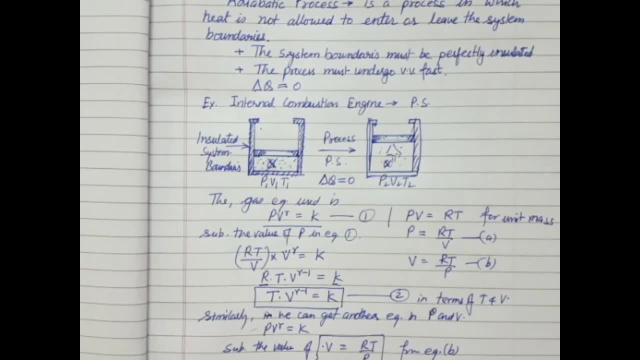 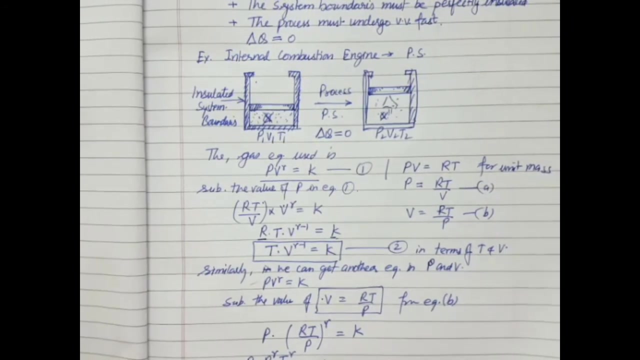 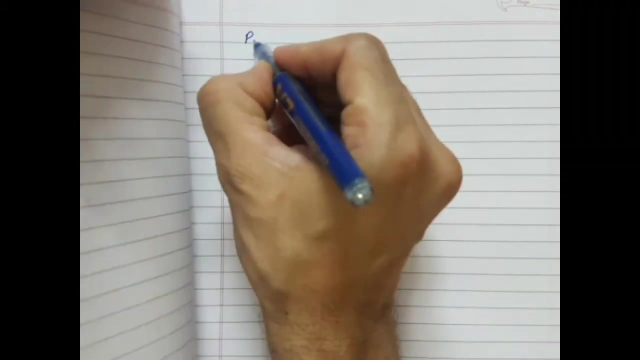 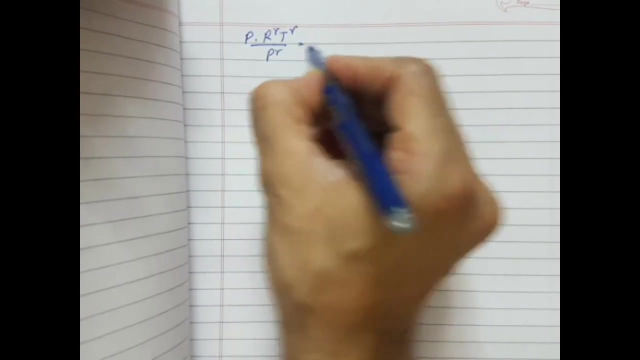 So again, P into R raised to power gamma, T raised to power gamma Divided by P raised to power gamma is equal to K. Go very down. So move on to next page. P times R, gamma, T, gamma over P raised to power gamma is equal to constant. so from here, 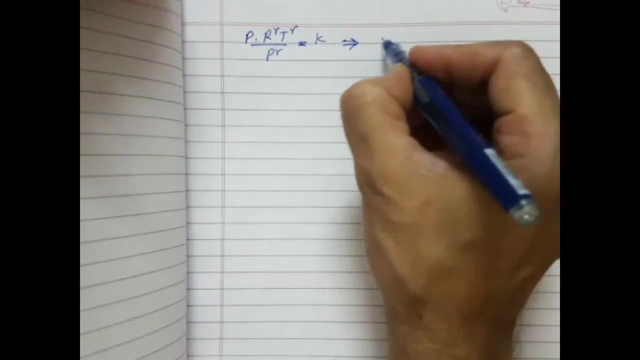 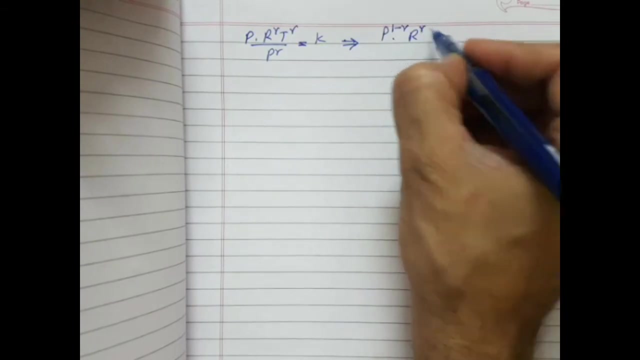 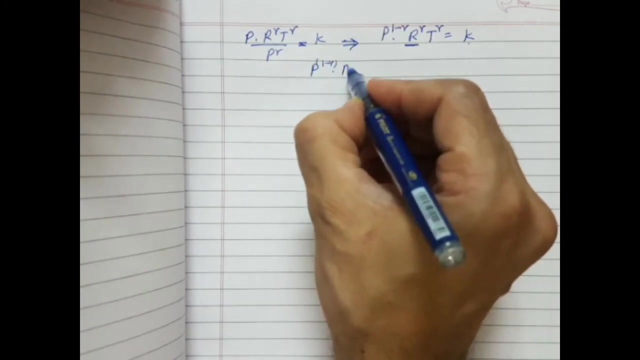 We can rewrite this equation as: P 1 minus gamma Into R- gamma T gamma is equal to constant. now here R is constant, so we can rewrite this equation like: P 1 minus gamma Into R- solid T gamma is equal to constant. So this is another equation. 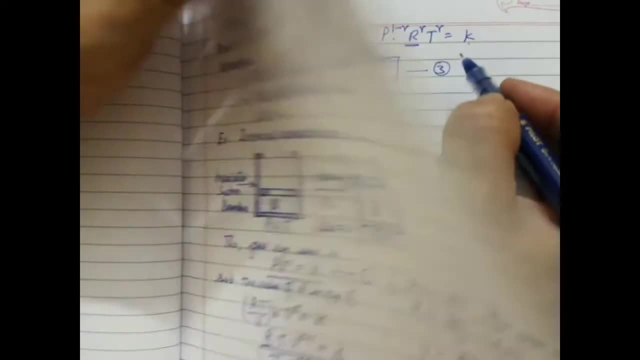 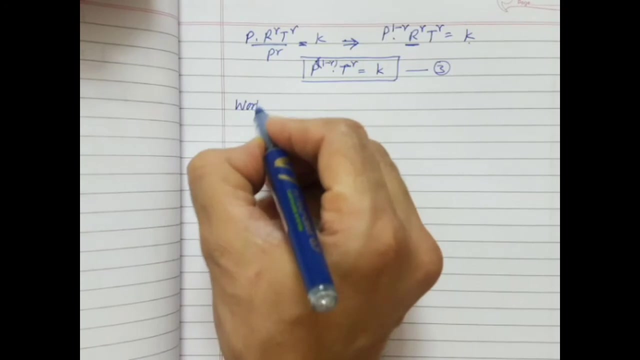 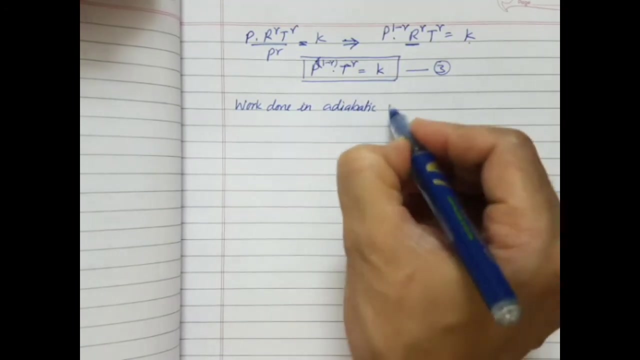 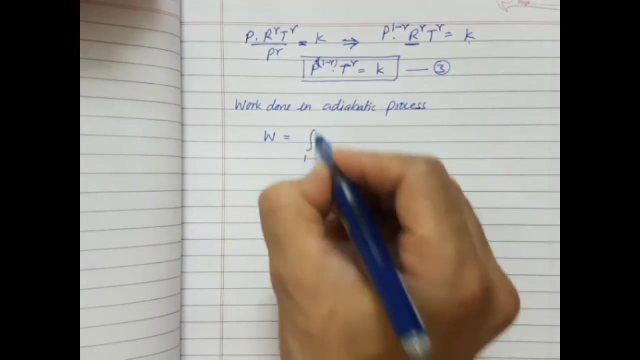 In terms of pressure and temperature. equation number 3: Yes. Now let us calculate the work done. now, work done In an atmospheric process. Now we know that work done is equal to 1 to 2 P times V DV. Now we know that in this equating, 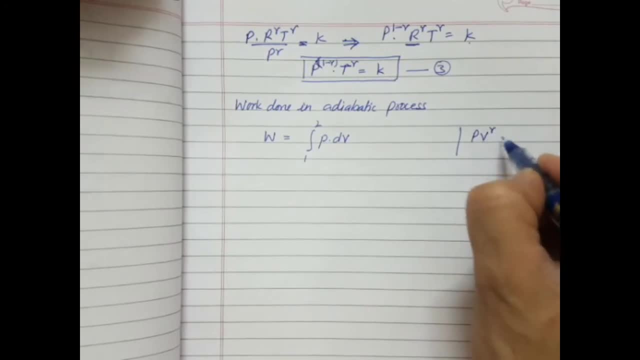 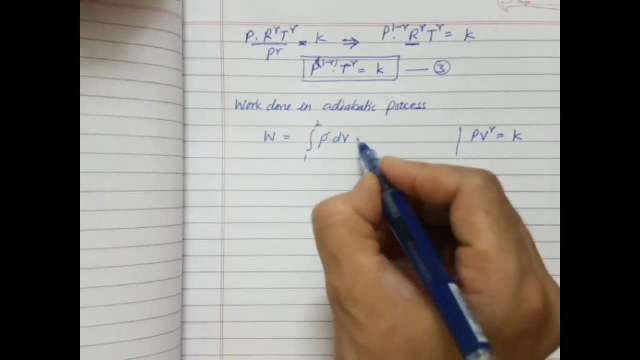 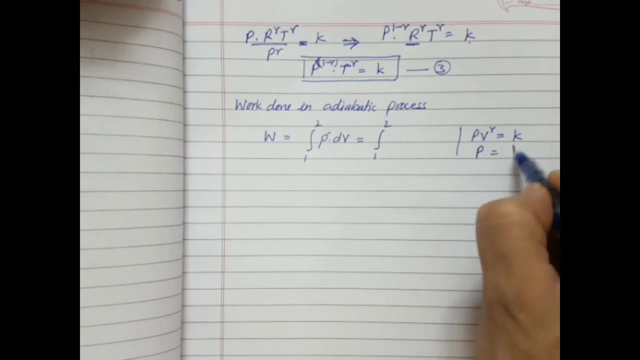 Adapting process. we have used this equation: P, V raised to power gamma is equal to constant, so We can substitute in the value of pressure Here, so we can write it as 1 to 2. Here P is equal to constant, So constant by V raised to power gamma. so 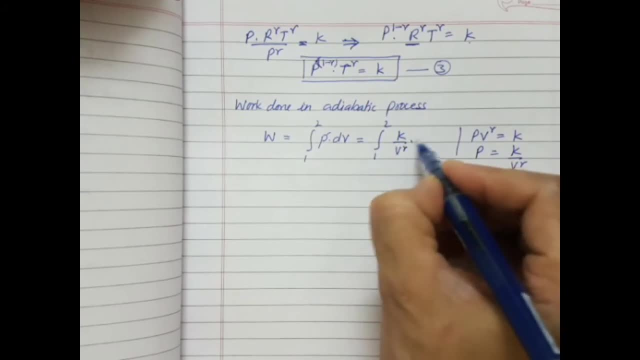 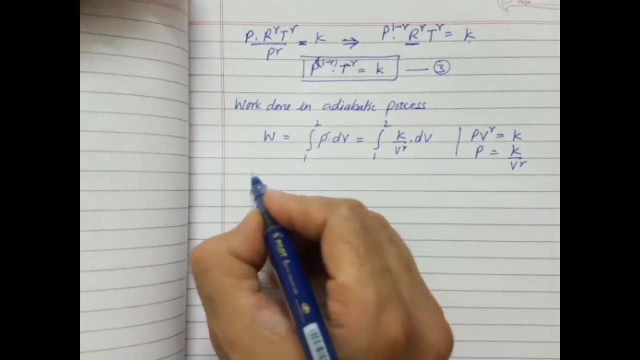 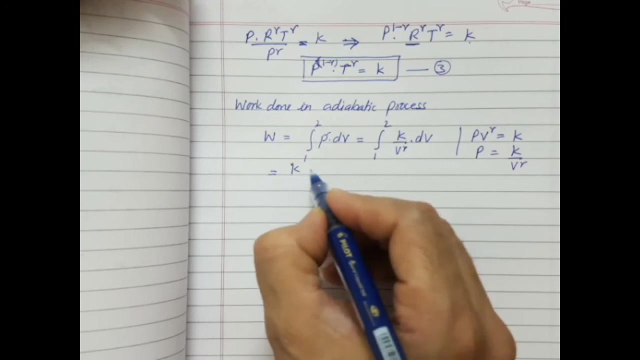 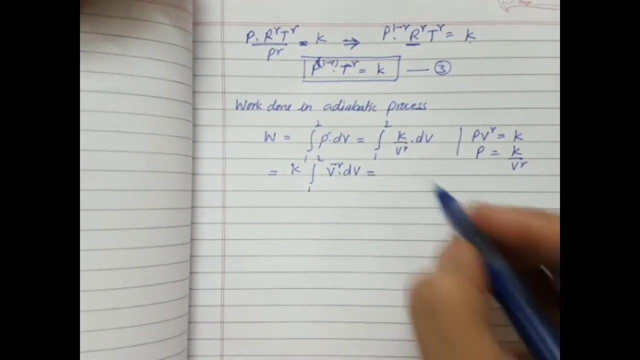 K by V raised to power gamma into DV. Now this is equal to K times 1 to 2 V raised to power minus gamma into DV. now integral of this is K times V raised to power minus gamma plus 1 over minus gamma plus 1. now this is equal to, you know, integral of. 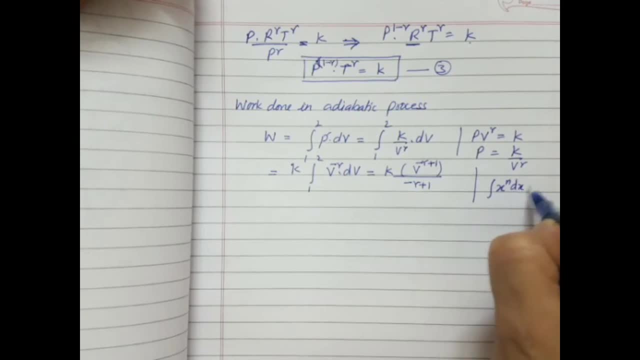 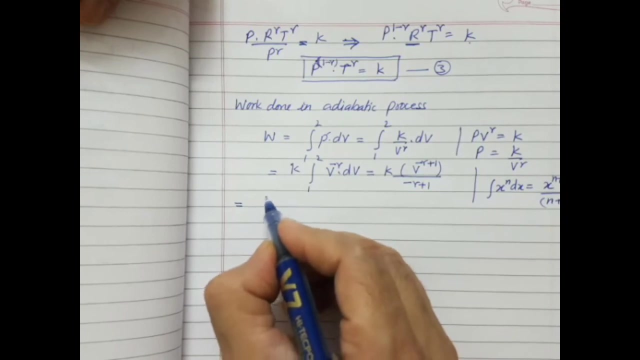 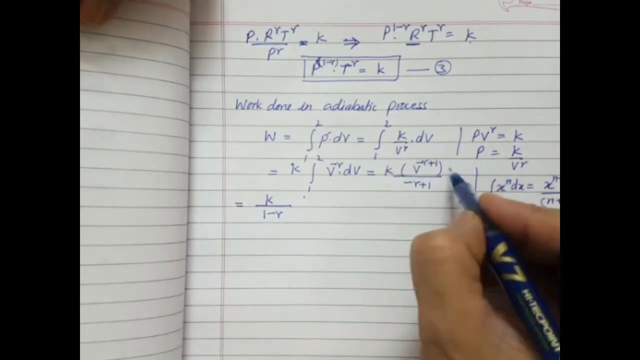 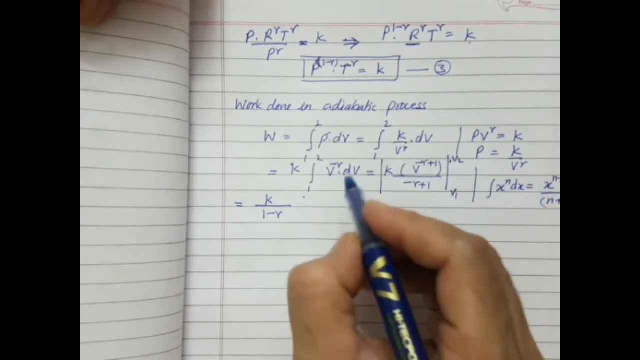 X raised to power n into DX. this is equal to X raised to power n plus 1. over n plus 1, We use this relationship. So here we ultimately we get Work done- is equal to k times 1 minus gamma in the bracket. Sorry, forget to take this v1 to v2.. So we get k. 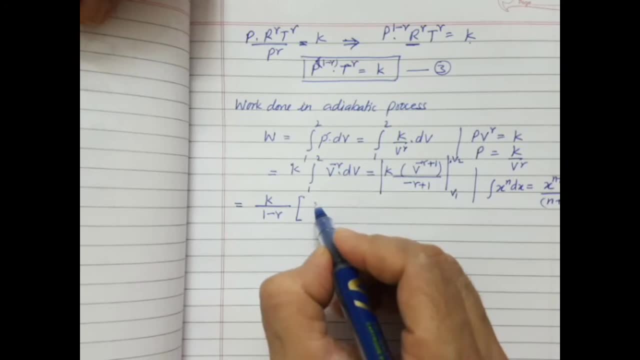 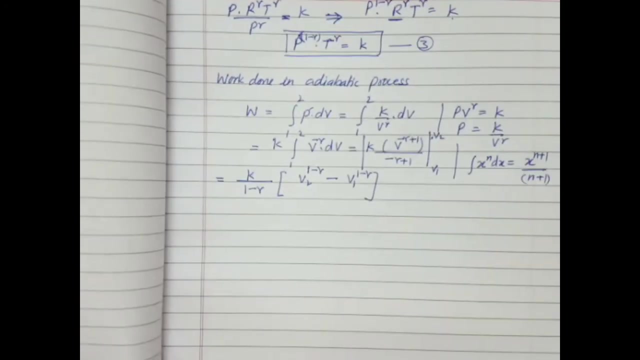 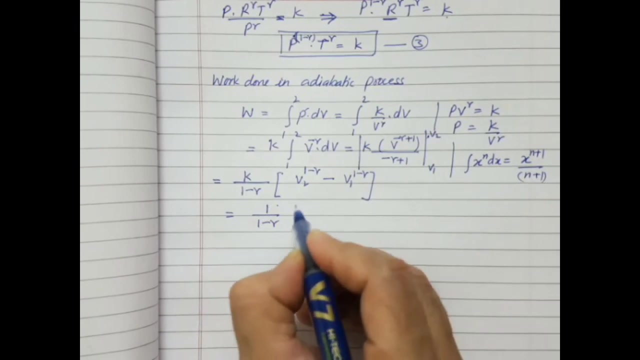 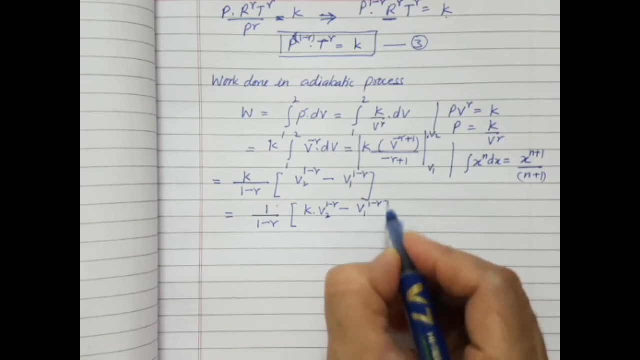 times 1 minus gamma. over in bracket We have v2: 1 minus gamma. We can rewrite this like this: minus v1, 1 minus gamma. Now again, we can rewrite this as 1 by 1 minus gamma. k times v2: 1 minus gamma minus v1: 1 minus gamma. Now we know that p1- v1 is equal to p2. v2 is equal. 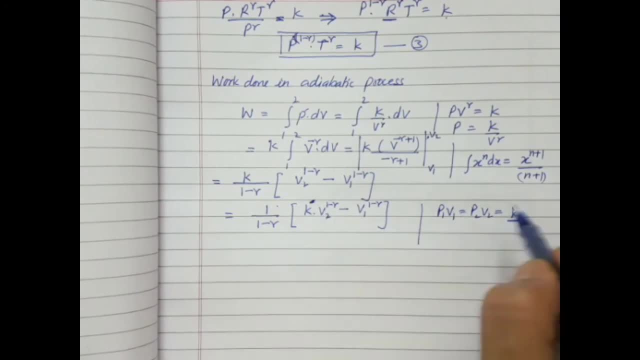 to k Now, substituting the value of k here From here now, k is equal to p1- v1 and k is also is equal to p2 v2.. So rewrite this equation like this: 1 minus gamma into p2, v2 into v2. 1 minus gamma minus p1 v1 into v1: 1 minus. 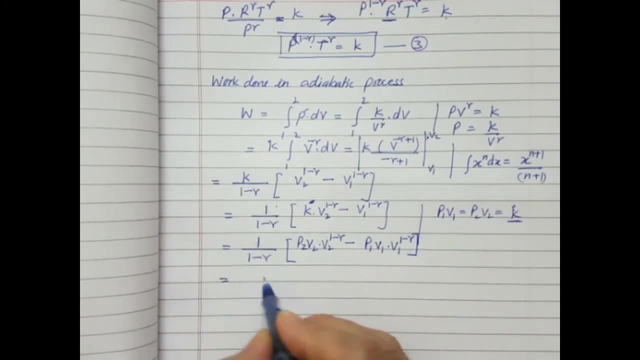 gamma. Now this becomes 1 by 1 minus gamma. Now v2 into v2, 1 minus gamma becomes 1 minus gamma, 1 plus 1 minus gamma. p2. sorry, here is there is gamma. p1. v1 gamma is equal to p2. v2 gamma is: